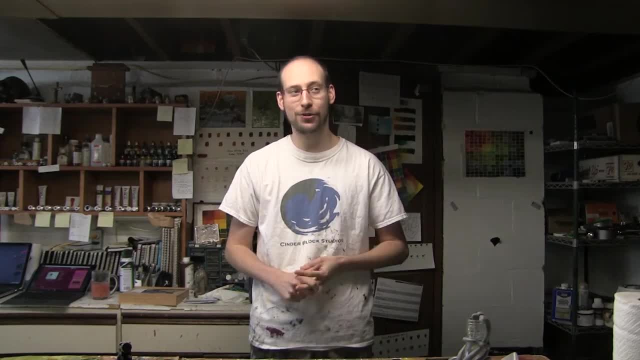 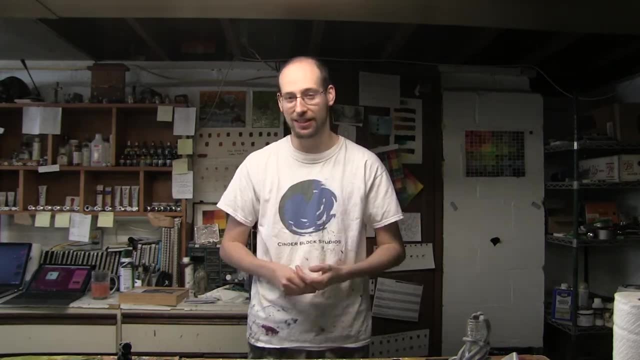 people's specific works, of the specific pieces, but you see what they're doing with techniques and grab those and then grab some from another artist, and then grab some from another artist. and when you mix them all together and adapt them into your own work, then that's usually. 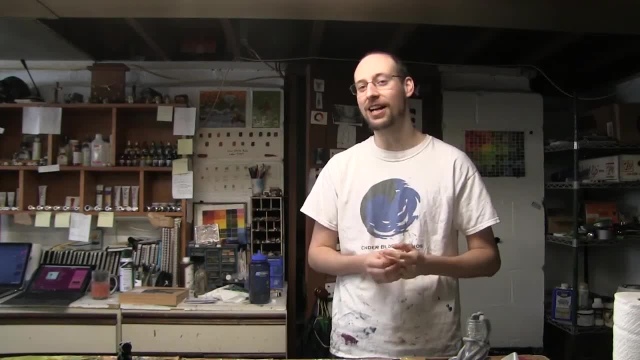 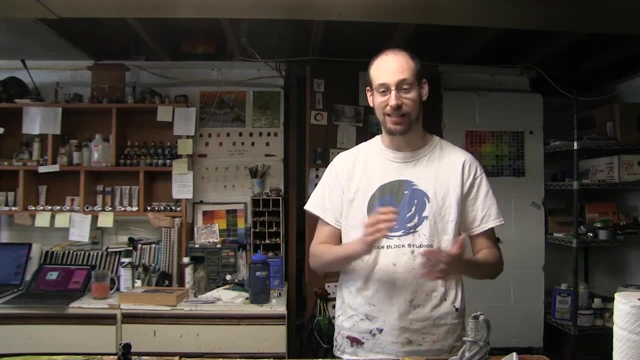 when people say, wow, you're really original. So today I wanted to look at five different techniques that I've sort of adapted into my work over the past ten years, and really they've been just from artists that I've found online And I was like, hey, this looks cool, I'm going to try it. I tried it and I pushed it. 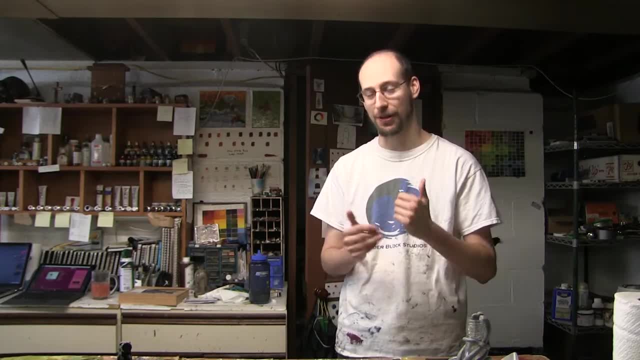 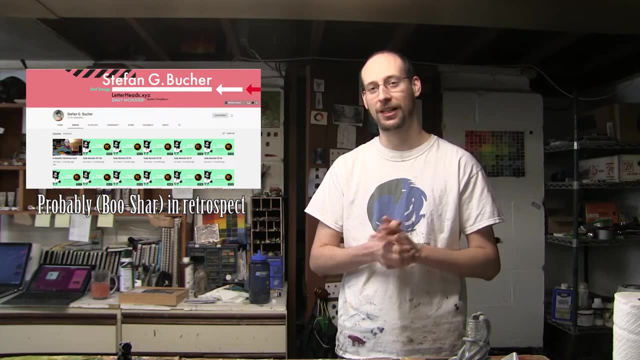 a little bit further and made it something more unique to my own using. So the first one is an artist by the name of Stefan Butcher and his ink spray technique from his YouTube channel, The Daily Monster. I actually found out recently the guy started uploading again. 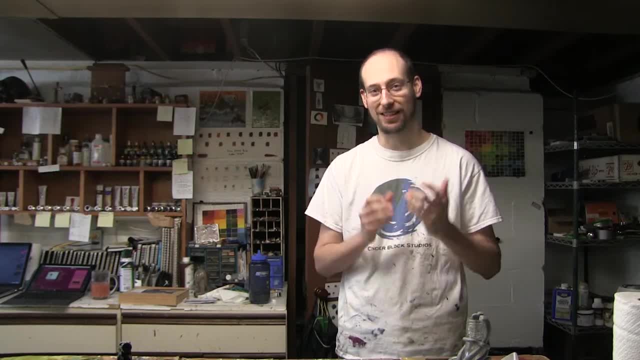 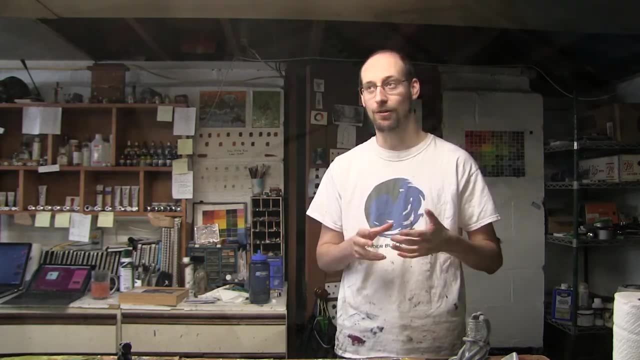 after a really long gap and I was really excited to see that, because I love the guy's work. What he does is he sprays, puts down a blob of ink, then grabs a can of compressed air, or what you might call a computer duster, and blasts that and it sprays out the ink in a 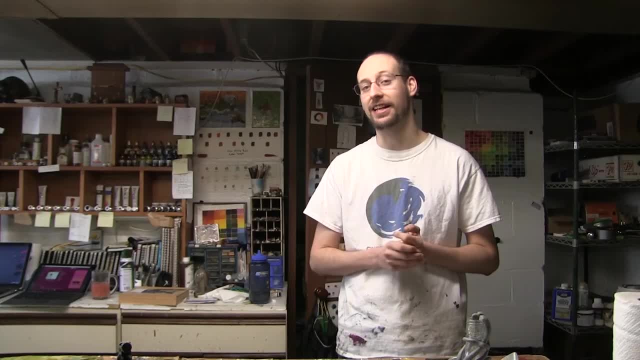 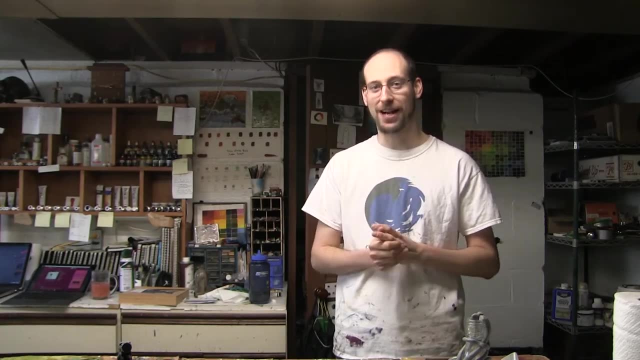 really unique pattern. It kind of branches out. Now, what he did with that technique is would do the spray and then draw like a creature around it. Given his graphic design background, it kind of was more suiting to that thing. But I love that idea and I remember dropping 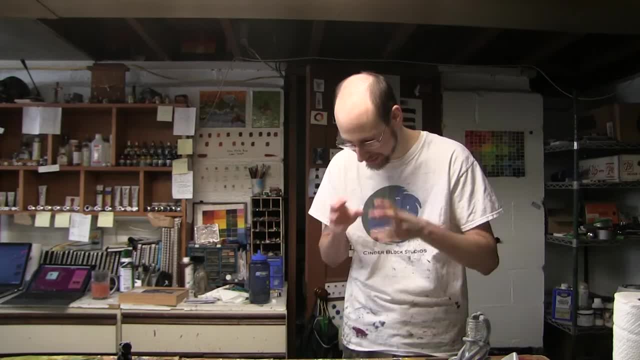 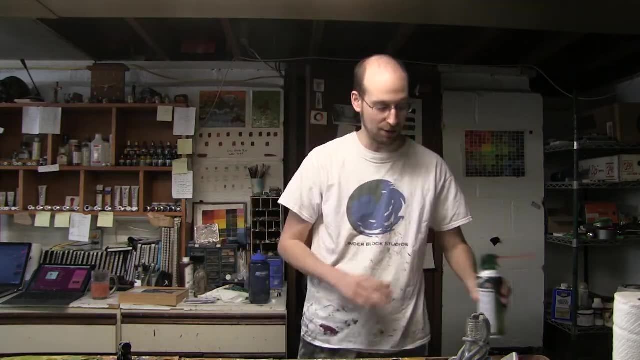 a comment back in the day, I was like, okay, what exactly are you using? Are you just sitting there and like blowing with a straw And he goes. no, I use a can of- you know- compressed air And I gave the ink a little one of those And I was like, oh man, that is brilliant. 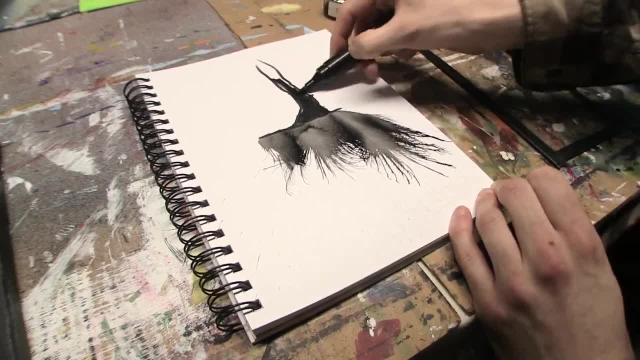 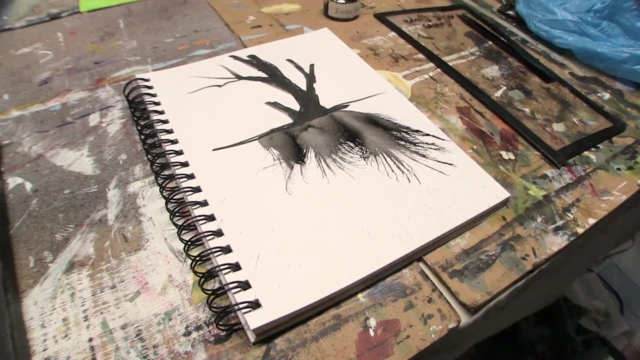 So I started doing that. But rather than creating a monster around it, it looks like a bunch of weeds or like a root system. So I'd flip the whole thing over and draw a tree on top of it, and it actually looks pretty awesome. The second technique I grabbed was by an artist. 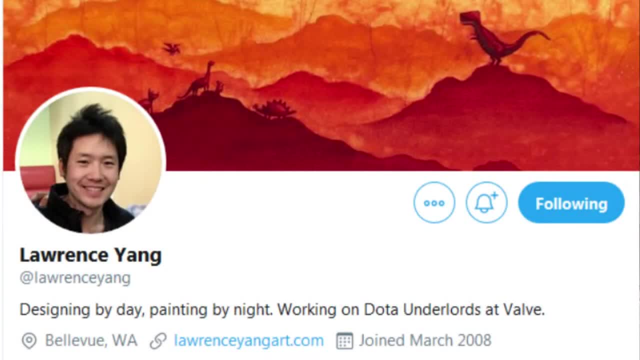 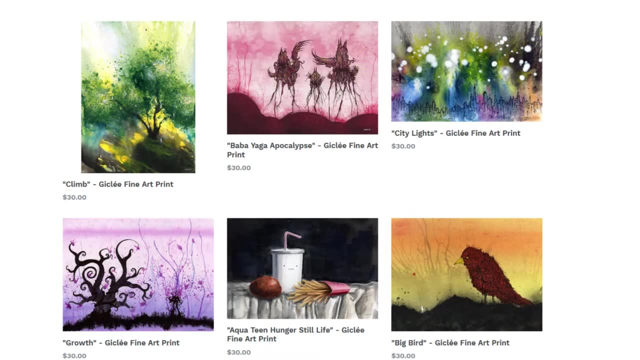 by the name of Lawrence Yang. I've been following his work since college and I've talked about his stuff on this channel here before, But what I kind of saw with him is just a layering technique with mixed media, something I at that point in time had never really seen before. 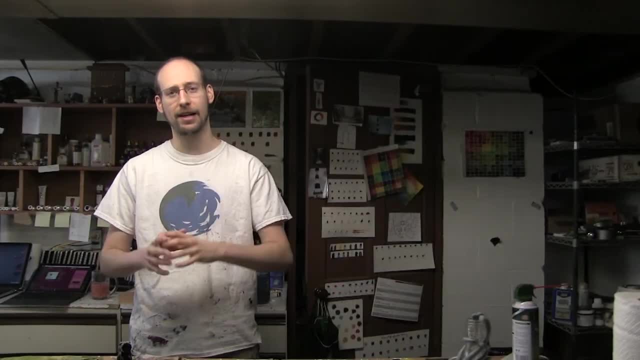 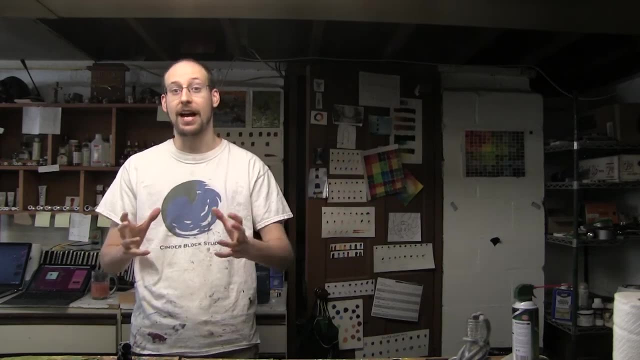 He primarily uses watercolor and gouache in the background and then comes on top of that with ink. Back in 2010,, I actually essentially copied that and, just like, let's just do watercolor, and I didn't have a whole lot of ink around at that point in time, So I just thinned out. 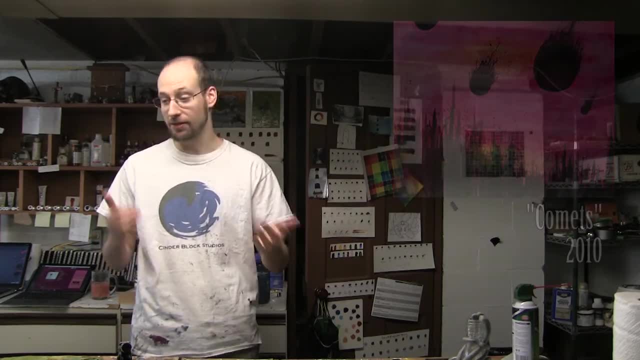 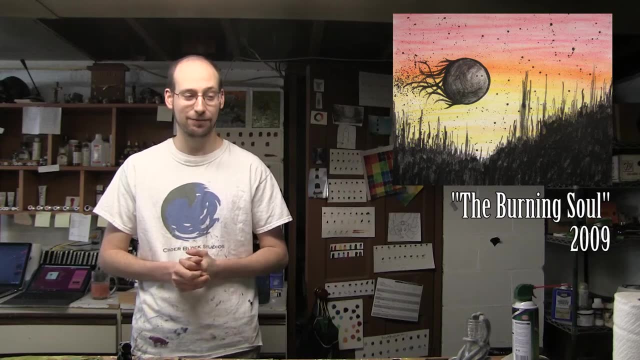 black acrylic and was using that, And some of those pieces, despite being 10 years old, of my own collection, are still some of my favorite pieces I've ever done And I still incorporate some of those techniques today in some of the things, like my watercolor book. 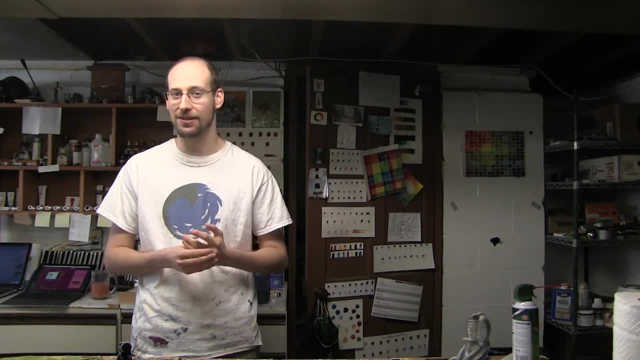 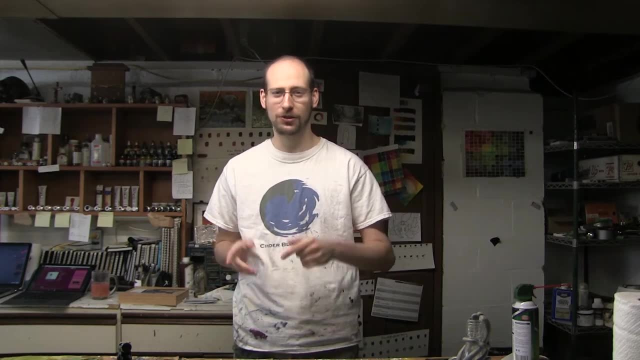 watercolor bookmarks and small print pieces and things like that that I'll sell in my print box when I go to shows. Next up is a technique that I've actually talked about, I think, at least once or twice here before, at least on a live show as well as over on. 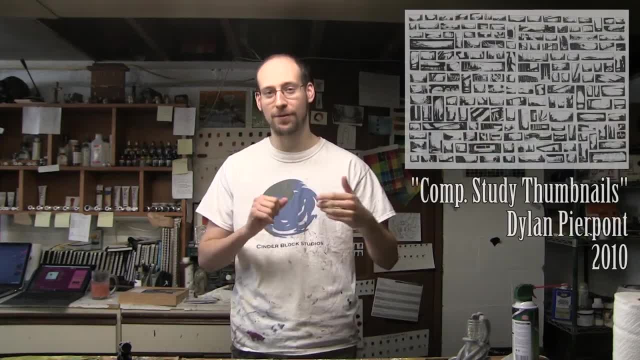 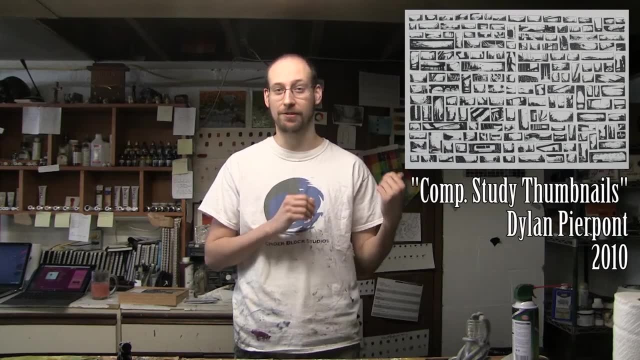 my second channel Sketch Every Day and it's the mini thumbnails. I picked this up from a guy by the name of Dylan Pierpont. He actually is a working artist out in, I think, Seattle at Microsoft. I connected with him online sometime after. I basically stole the technique. 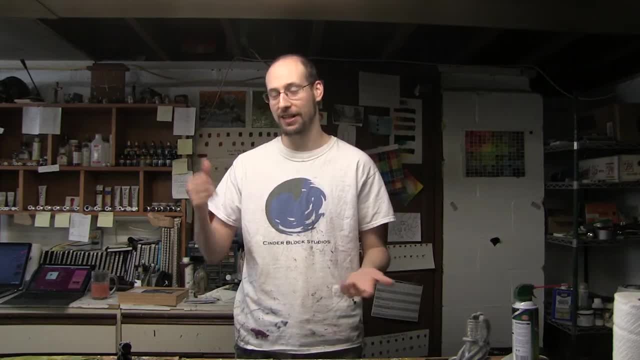 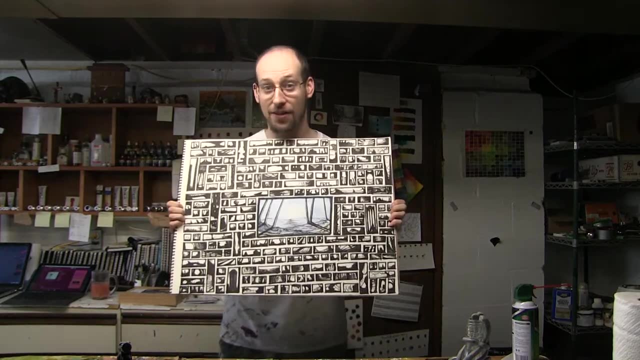 And then he told me that he just stole. he himself stole the technique from, like a teacher of his. So it's just an ongoing process. But I was so enamored and inspired by that I did this massive 18 by 24 sheet of paper and 208 little compositions using that technique. 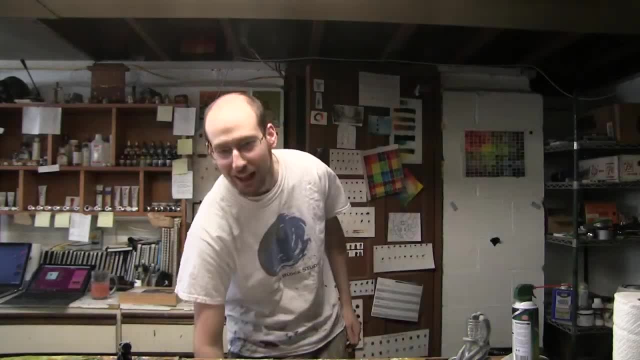 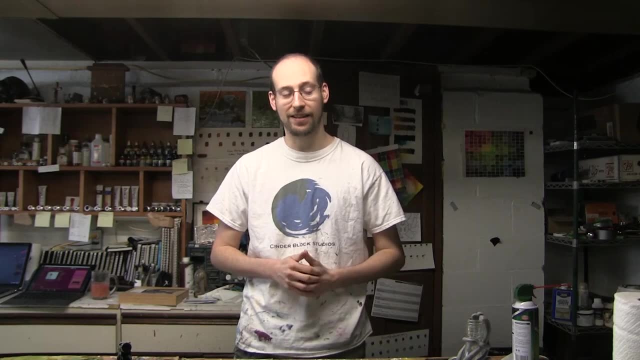 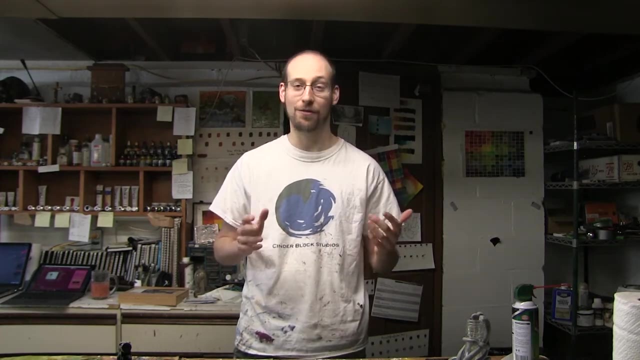 You can see a time lapse of this over on my second channel. And I love the technique so much and I really learned so much from it, that I literally adapted it straight into my daily sketches And ever since that point in time I have used that technique almost every single day in order to create a lot of the work that 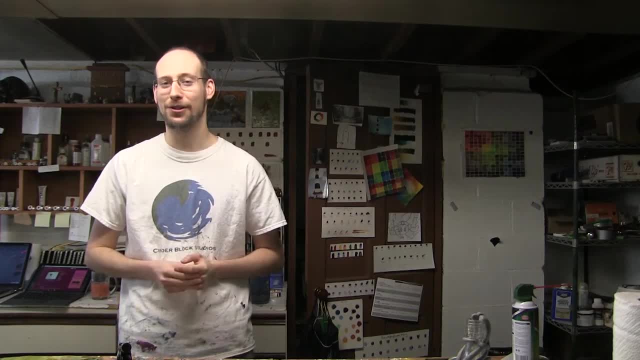 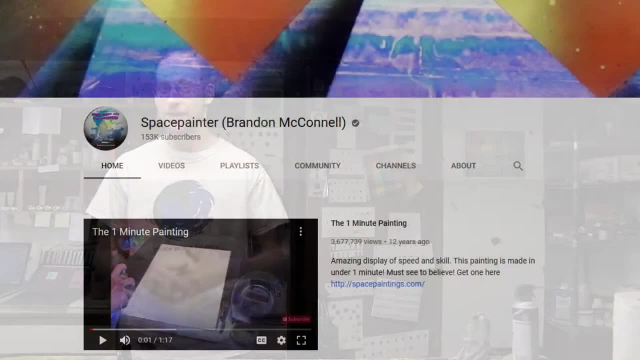 I've done over the past few years. Next up, for anyone who's been on YouTube a very long time, you might be familiar with what is known as the space painters, specifically a guy by the name of Brandon McConnell who kind of popularized this idea of quick 30 minute. 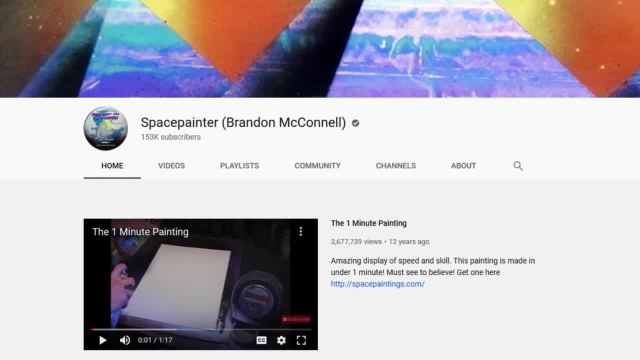 or even I think God he must have had like 30 second, one minute draw paintings. that he did. It was a lot of spray paint on like a piece of poster board and played with like newspaper. He got this really great layering technique and like flicked it all over the. 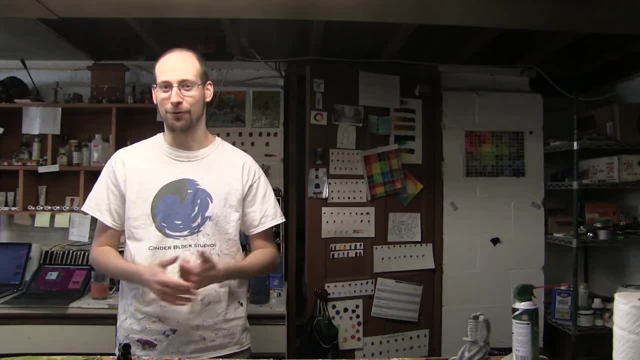 space And it's a really cool technique. And it's a really cool technique And it's kind of like flicked stars in. There's a lot of techniques I actually pulled from watching those videos, But the one that I really kind of took to heart was just using spray paint. 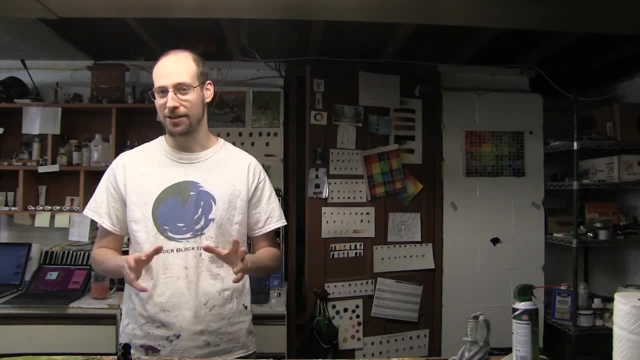 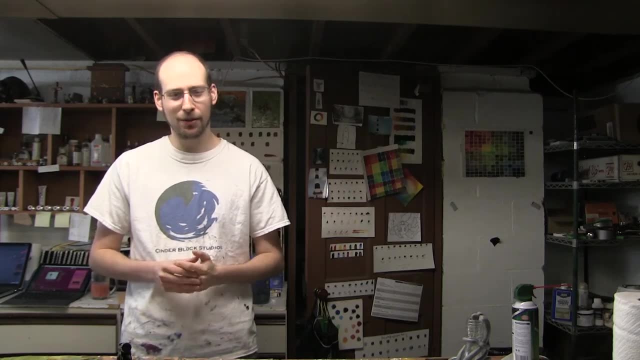 on canvas. Now I tried my hand at a couple of these little space paintings and I was nowhere near as good at it as he was, obviously because I just started doing it, But I was like you know what I'm not. It's really inspiring, It's fun, It sells a lot at street. 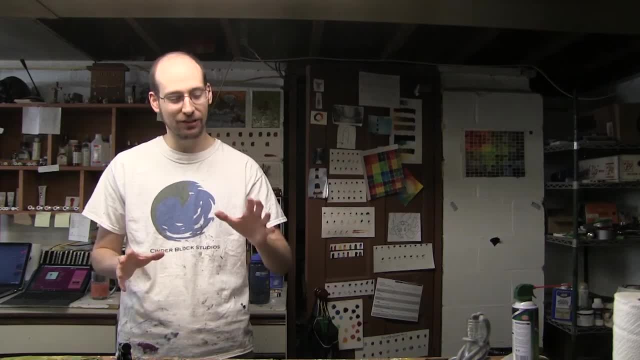 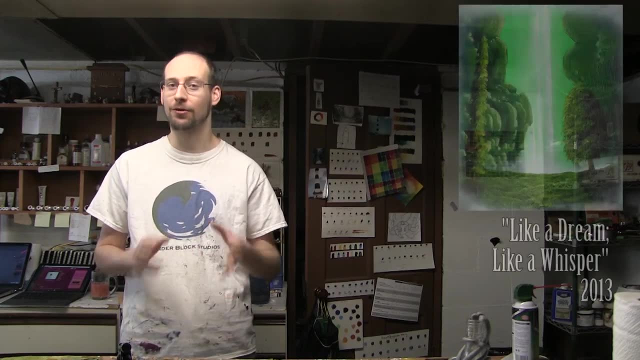 art shows and things like that. But I'm like you know, I like the idea of just trying to adapt something else in. So one thing I grabbed out of that was just using some white spray paint specifically to add mist and fog in my work, And ever since then I've been using it on a large number. 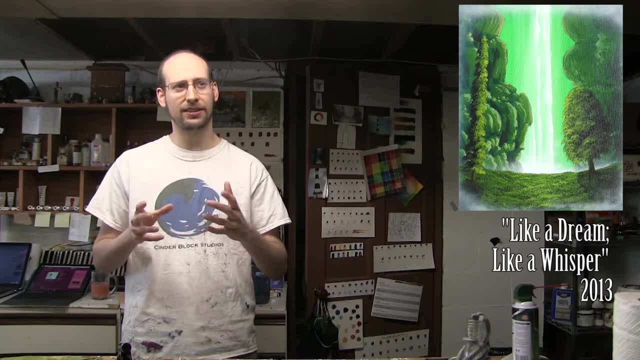 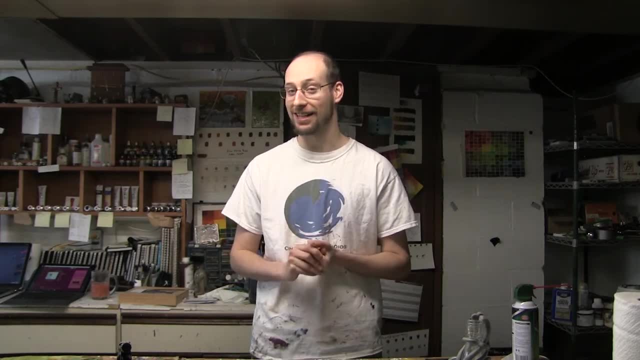 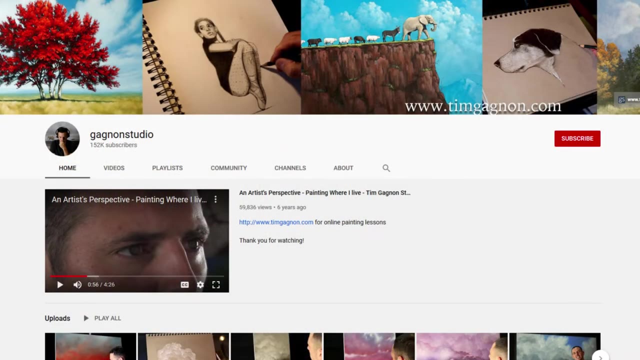 of pieces, to the point where, unless I'm doing a night scene or a space scene, I'm probably using it on almost every piece. And the last one is another fellow YouTuber, a guy that's been doing it just a little bit longer than I have, actually Tim Gonnard and his three-layer. 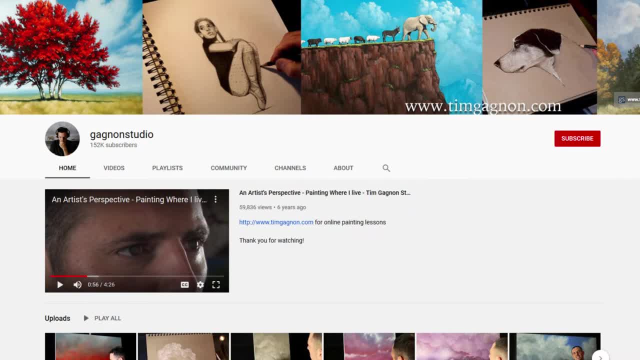 foliage technique. This technique is called the three-layer foliage technique And it's a little bit different than the three-layer foliage technique. This technique is called the three-layer foliage technique, If you look the guy up. I'll put a picture over here. 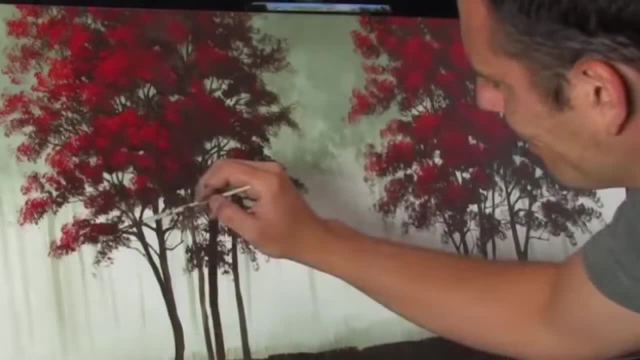 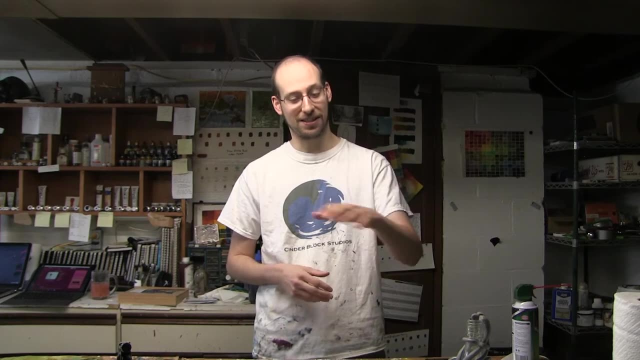 of the kind of stuff that he does And it's super inspiring one, because it's a very simple technique. It makes things a lot more realistic, And I sort of, along this era of all these other artists, discovered them around 2010.. And that was like the year that I sort 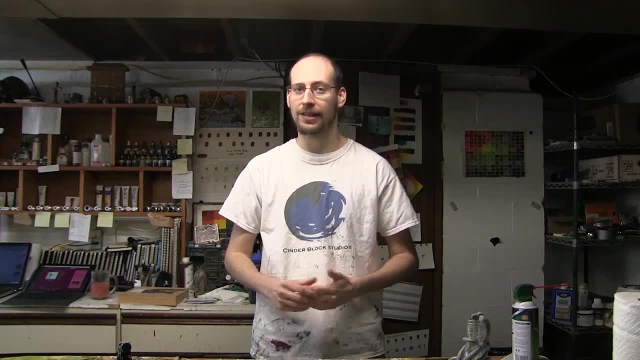 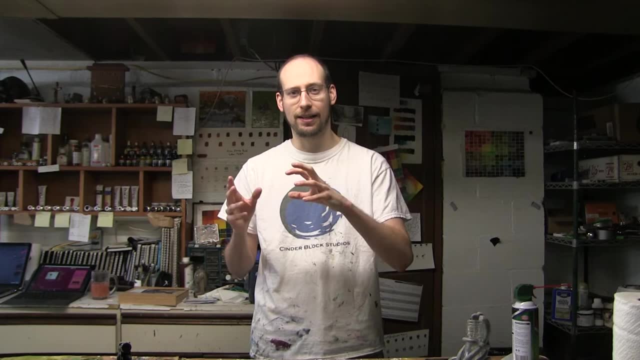 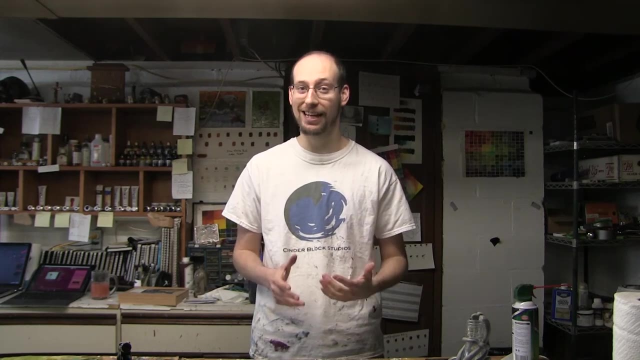 of really kind of jumping forward with my work and pushing my work further and learning a lot more techniques. Now I took the sort of three-level mid-tone, shadow and highlight design and actually created the vast majority of my current techniques. A large portion of what I do today is because of watching those videos and seeing how he worked and 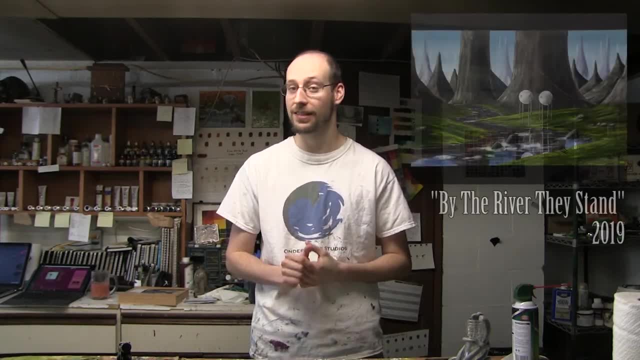 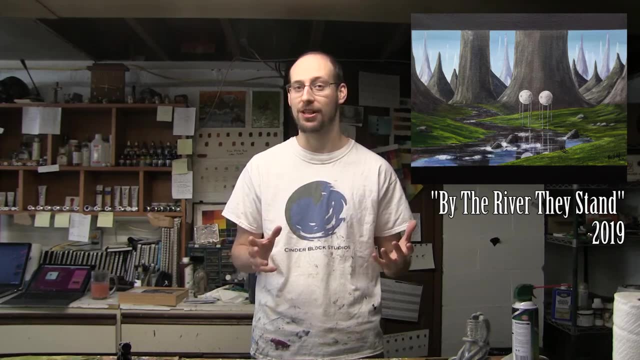 adapting that into my own work. Now, I don't necessarily paint as realistically as he does, but I use that same level of three distinct tonal values in order to create, like 99% of the work that I do today. So, when it comes to being inspired by other artists and other, 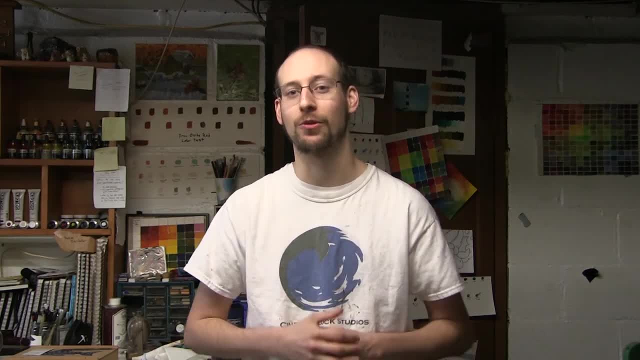 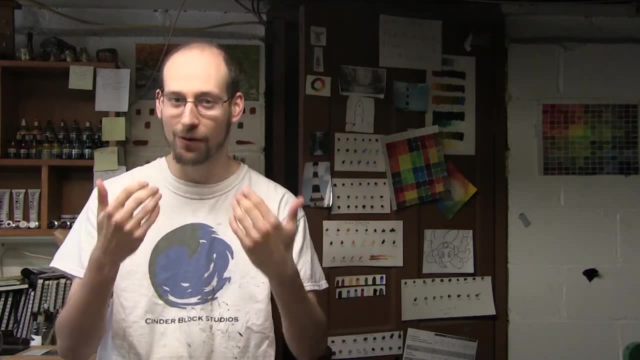 techniques. it's important to use those techniques in your own work to build up your own working. set In trying new techniques and trying new ideas and pushing them into your own work and adapting them, just however they decide to work for you. it's like this is how you. 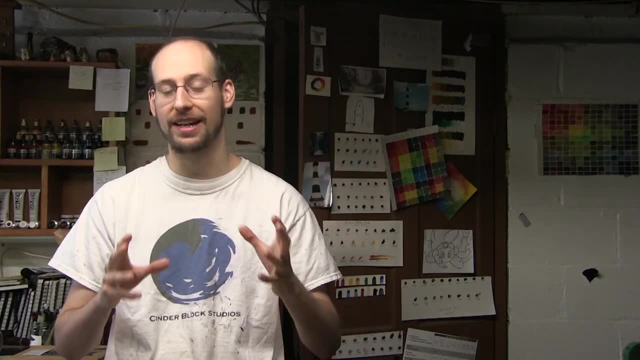 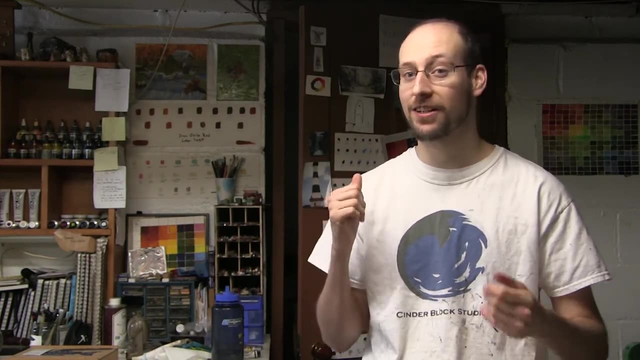 develop one new techniques for yourself, as well as to further your work in new ways. As an artist, it's always important to really kind of push your limits And, if you don't know where to start, grab a technique that another artist is using and just play with.